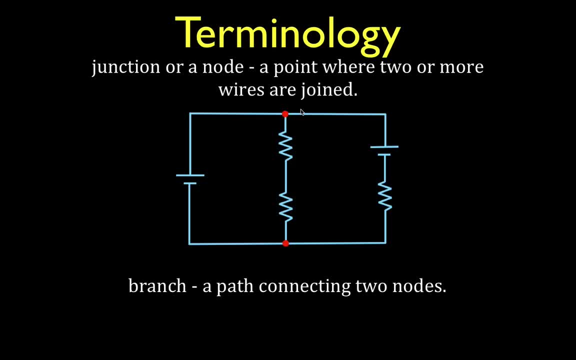 and you can see, in this circuit we have node number one and we have another node down here. This is the place where the wires come together. Now, the branch is a path that connects two nodes and we have three branches. We have this branch that connects these two nodes. we have this branch. 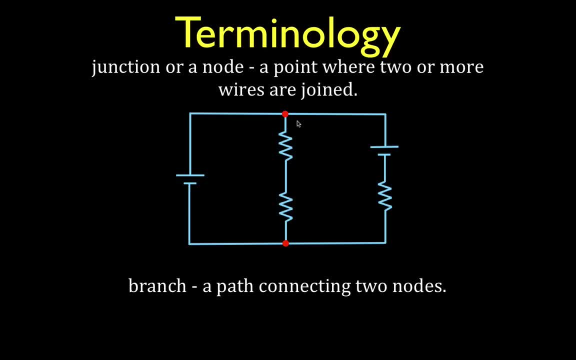 that connects these two nodes and we have this branch that connects these two nodes. So please don't forget that. So please don't forget that. So please be aware that you should know what a node is and be able to identify the nodes, what the branches are and be able to identify the branches. 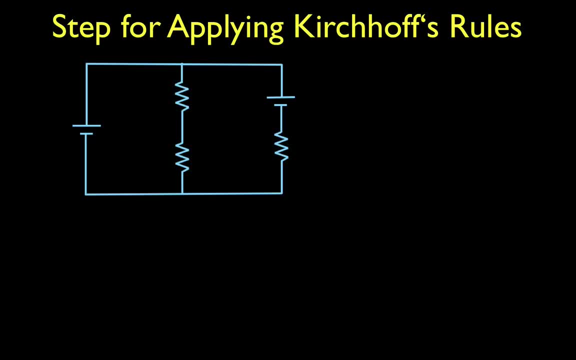 These are the steps. I would say there are five steps to applying Kirchhoff's Rules. The first three are really things you do before you apply the rules. Step four and step five are applying the current and the voltage rule. The first thing you should do is label the nodes, Identify and label them. 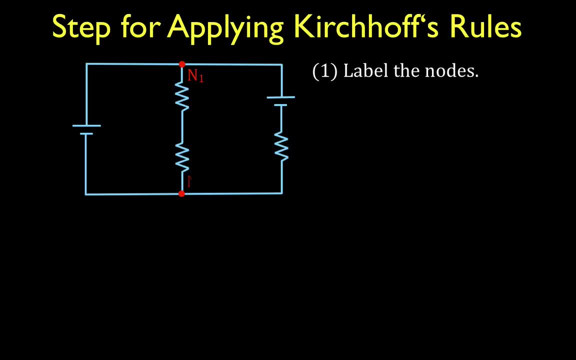 There's one, We'll call that N1.. There's that one, We'll call that N2.. Now the next thing we're going to do is we're going to assign a current and a direction of the current in each branch. 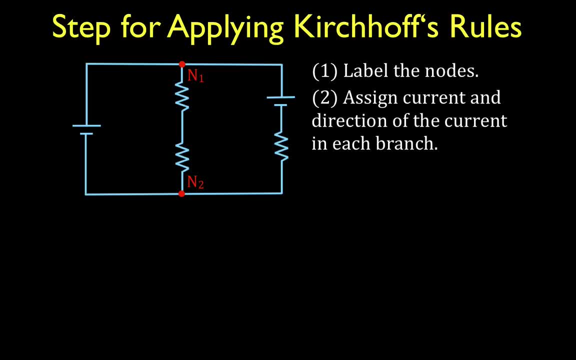 I would like to say quickly that the direction we choose is completely arbitrary When we calculate the currents. if we get a positive answer, we'll know we chose the correct direction. If we get a negative answer when we calculate the current, it doesn't mean the current is negative. 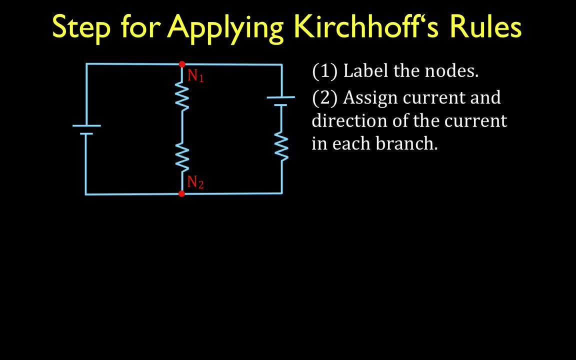 It only means that we chose the wrong direction for the current. So I have three branches. The first branch I'm going to say is this one on the left-hand side, That is a current which I'll identify as I1, and it's basically going clockwise. 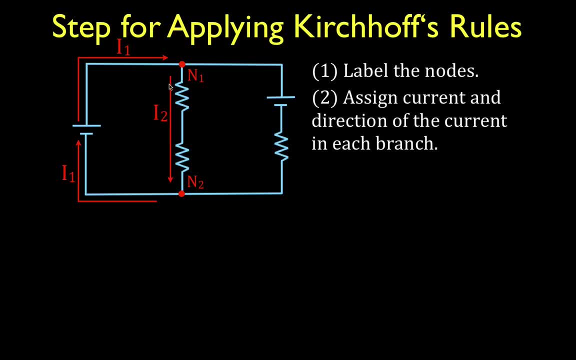 The second current I2,, we'll say, goes from top to bottom between these two nodes. The third current I3, goes on the right-hand side here and it flows clockwise in this direction also. So we have current one, current two and current three. 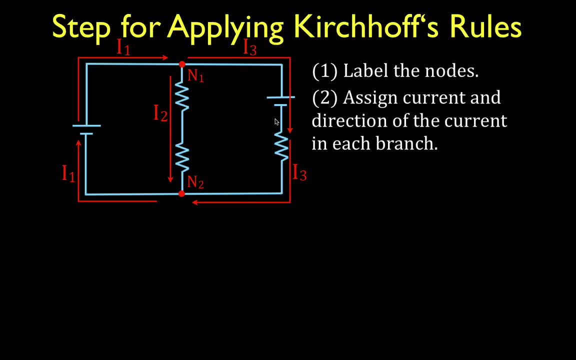 Each branch has a current. Now, before we go on, I just want to say that when we apply Kirchhoff's rules and the current, what we're finding is the conventional current, which is the flow of positive charge. The electrons actually flow in the opposite direction. 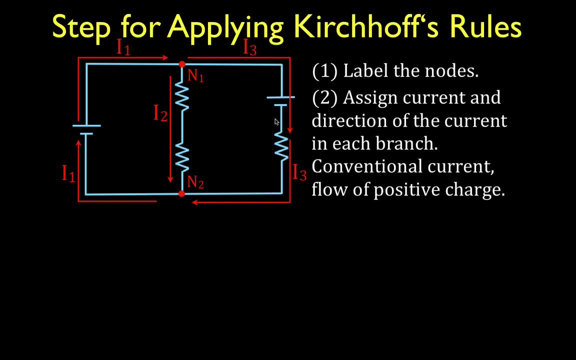 But this is for conventional current, which is the flow of positive charge. Okay, these are the two things we did so that we can apply the current rule. Now we have to do one thing So that we can then apply the voltage rule. 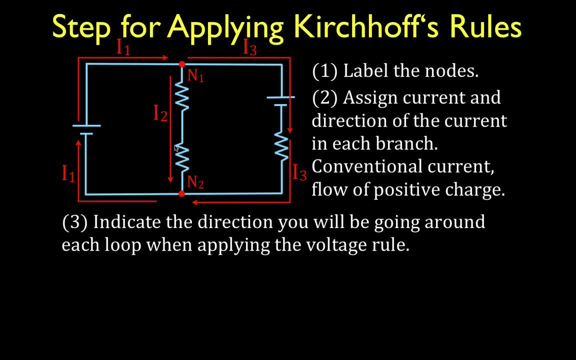 We have to indicate the direction that we will be going around each loop when applying the voltage rule. Now, the easiest thing to do, I think, is to just choose clockwise and clockwise. We have two loops, Loop one. we're going to go around clockwise. 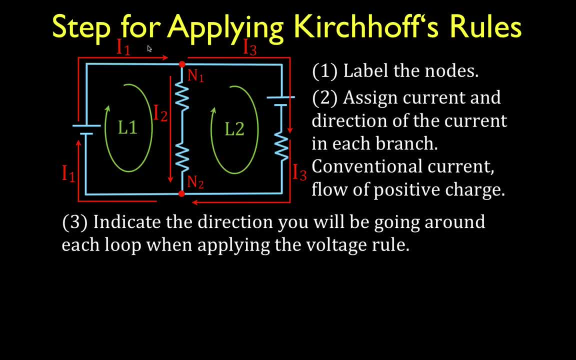 Loop two: we're going to go around clockwise. We could also say: all the way around the outside is loop three, But for this video we'll just talk about loop one and loop two, And we're going to do them both, Both clockwise. 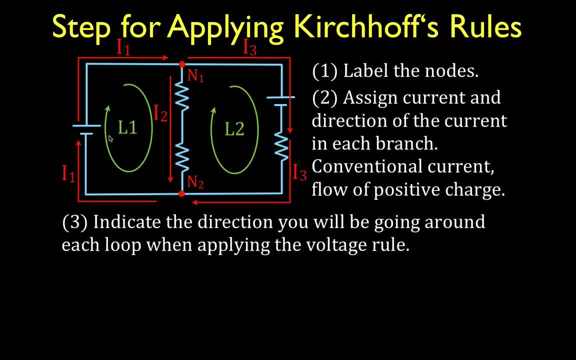 Now, once again, when you assign the direction of the current, it's arbitrary. When you assign the direction that you're going to go around each loop, when applying the voltage rule, it's also arbitrary. I chose clockwise and clockwise. You can choose counterclockwise for both of them. 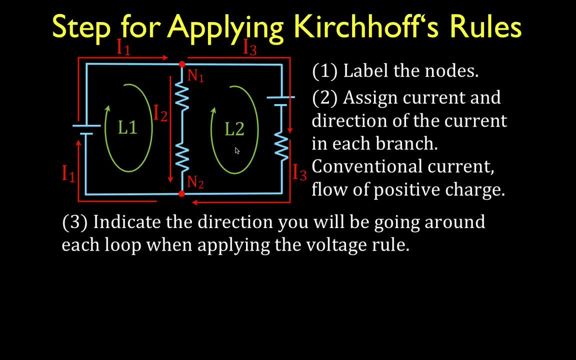 You can choose one counter and one clockwise, One clockwise and one counter. It doesn't matter, It'll come out in the math when we get the sign of the current Okay. Okay, step four is we're going to apply the current rule. 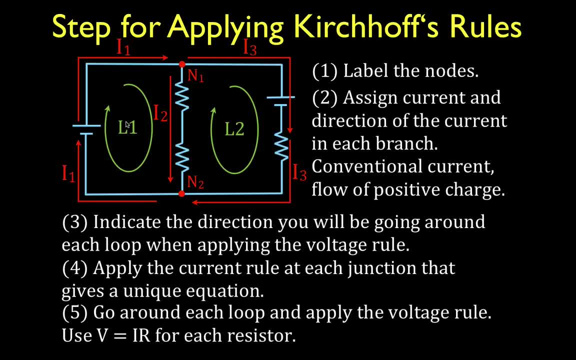 And then step five is we're going to apply the current rule. We're going to apply the voltage rule and use: V equals I times R at each of the resistors. Okay, So steps one through three are really the things you do before you apply the rules. 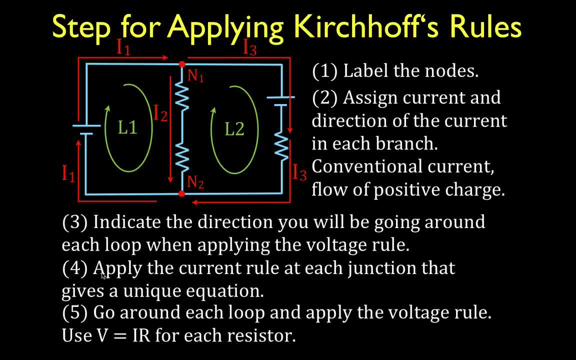 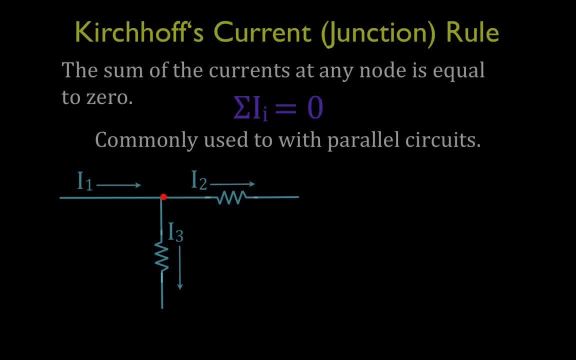 And then you apply each of the rules, And now in the next slides, I'm going to go through some particular things you need to keep in mind when you apply the current rule and when you apply the voltage rule. Okay, this is for the current rule. 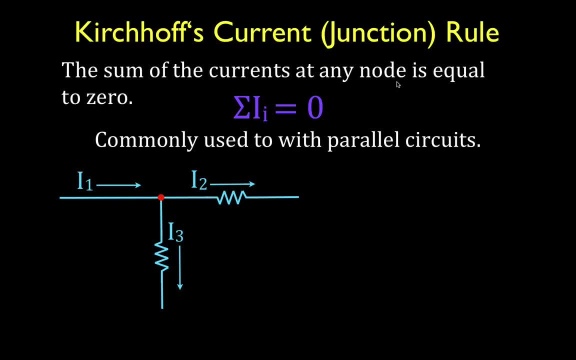 Kirchhoff's current rule says that the sum of the currents at any node are equal to zero. This says the sum of the currents is equal to zero, And this is something you should be a little bit familiar with when you've talked about just regular old parallel circuits. 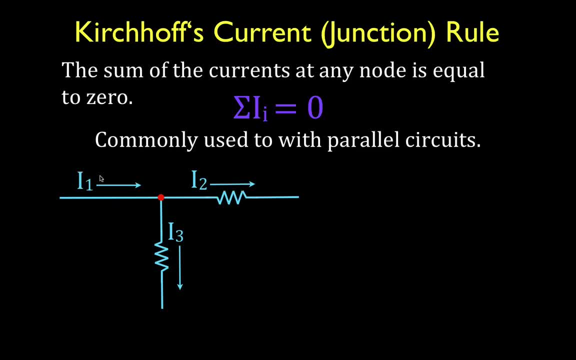 The sum of the currents at any node is equal to zero. That means if we sum up these three currents- because here is our node, we have one current in and two currents out- they have to be equal to zero. The current that comes into the node is commonly designated as positive. 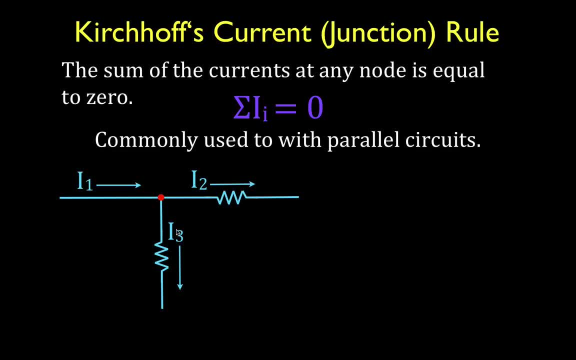 The currents that leave the node are commonly designated as negative. So when I sum up the currents for this node, I could write down that I1, which is positive, minus I2, minus I3, equals zero. This is the sum of the currents into the node. 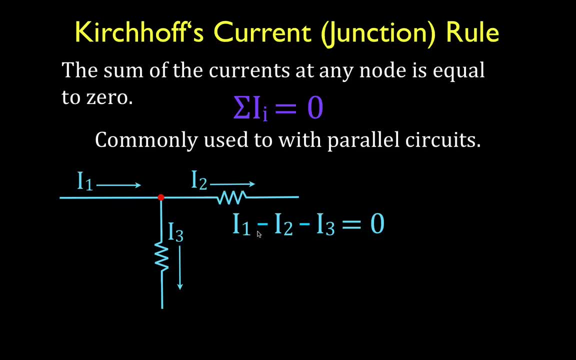 The sum of the currents at any node is equal to zero. Now you will often hear people say that the currents into the junction are equal to the currents out of the junction. That means the current in is I1.. The two out are I2 and I3. 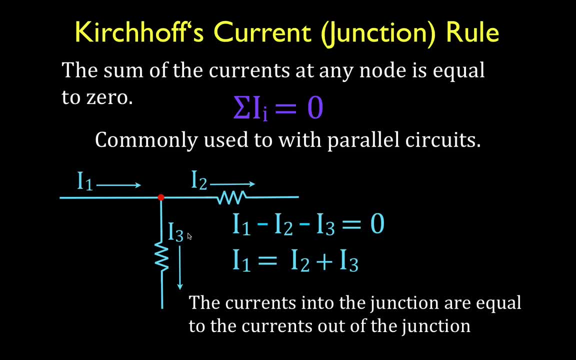 And we could write down that I1. The current in is equal to the currents that leave the junction I2 and I3. Now this equation and this equation are the same equation. I could simplify this. or if I just move I2 and I3 to the other side, I would get that I1 equals I2 plus I3. 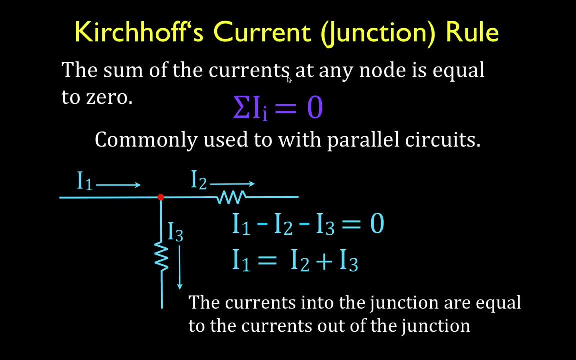 Okay, so there's kind of two different ways you can think about it. The sum of the currents is equal to zero, or the currents in are equal to the currents out. Okay, that is how you apply the current rule for Kirchhoff's laws. 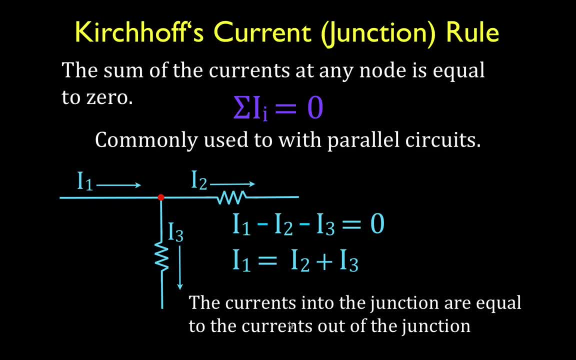 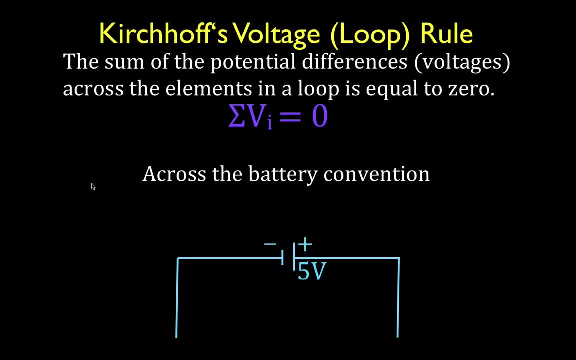 Okay, Now there are two things we need to be aware of when we apply the voltage rule. In both cases it says: the sum of the potential differences across all the elements in a loop is equal to zero. The sum of the voltage drops and gains is equal to zero. 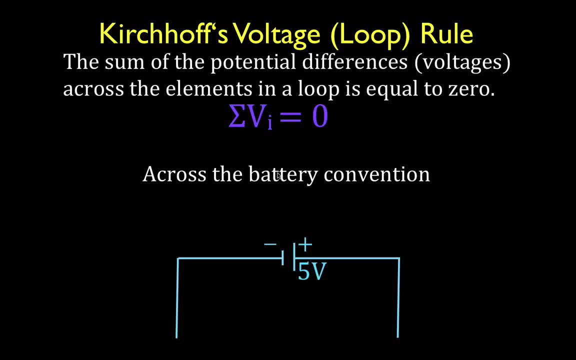 This is the cross the battery convention. We're going to have batteries and resistors in this video. Okay, Now cross the battery. If, when we go across the battery, we go from negative to positive, that's a potential increase. 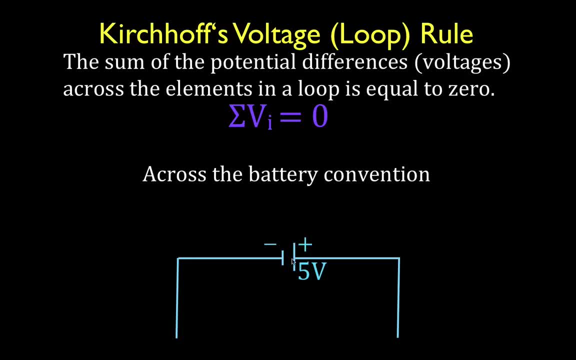 So if we had said that we're going to go around this loop clockwise, we would be going across the battery in this direction. That means we would have a voltage gain and we would write down plus five volts. Now, if we had chosen to go around this loop in the counterclockwise direction, 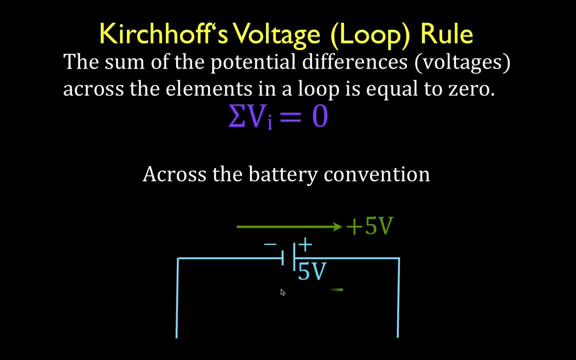 then we would be going across the battery in this direction. Okay, In this direction. when we sum up the voltages And we go from a positive to a negative, from a potential high to a potential low, then we would write down negative five volts. 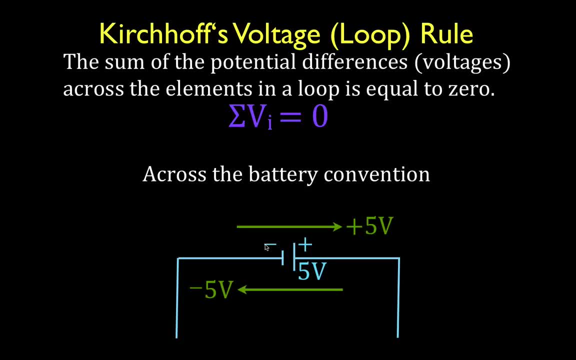 So you have to pay attention with the direction you're going across the battery, whether it's a potential gain or a potential decrease. All right, That is the battery convention. Now we have the resistor convention. Now this one looks a little bit more complicated. 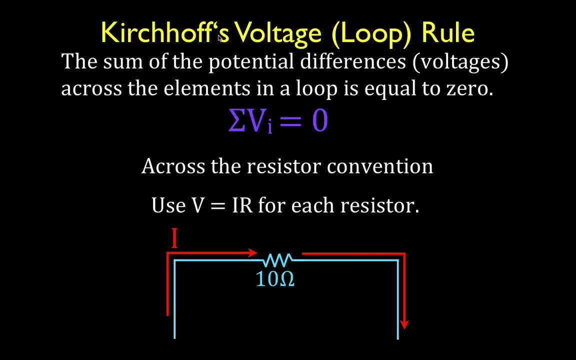 But it's basically this. But it's basically the same thing, because it's also Kirchhoff's voltage rule. The sum of the potential differences across the elements in a loop is equal to zero. The sum of the voltages is equal to zero. 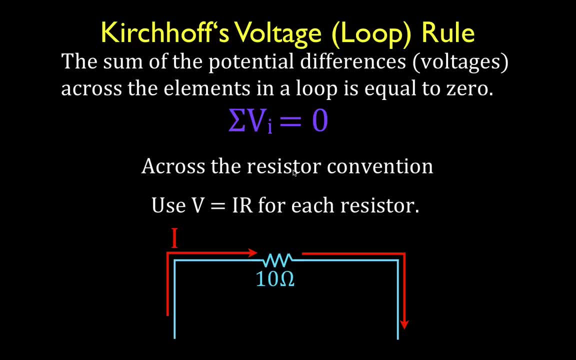 This is the resistor convention. We're not going to a resistor convention, but this is the resistor convention. Okay, Now we're going to use V equals I times R. Here is I indicated the current direction we chose for this branch. 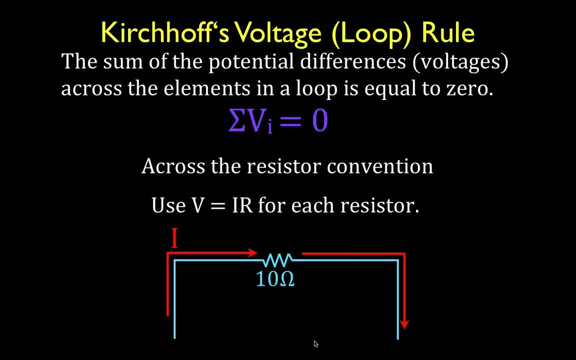 Now, once again, if we go around this loop in the clockwise direction, we would be going across the resistor. in this direction, That means we'd be going with the current. When the current flows through the resistor, it loses energy And therefore the potential difference across this resistor. 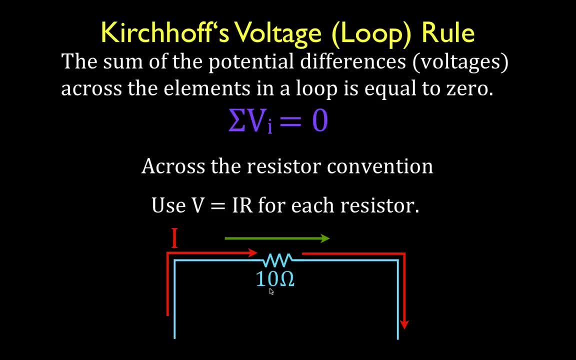 is equal to the current times, the resistance, And we say that it's negative, The current times, the resistance. I times R V equals I times R Ohm's law. So, but we put a negative sign because we're going with the current in this case. 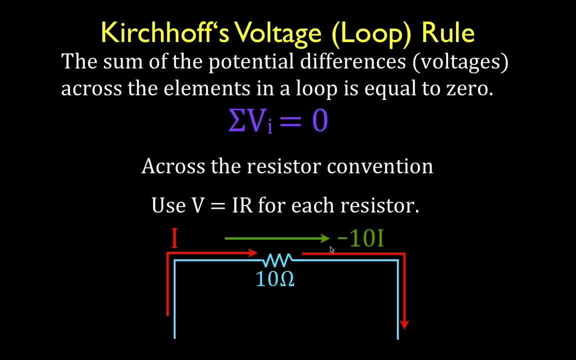 And therefore there's a potential decrease. Now, if we had chosen in this loop to go in the counterclockwise direction, then when we go across this resistor, we would be going in this direction, which is against the current or upstream. 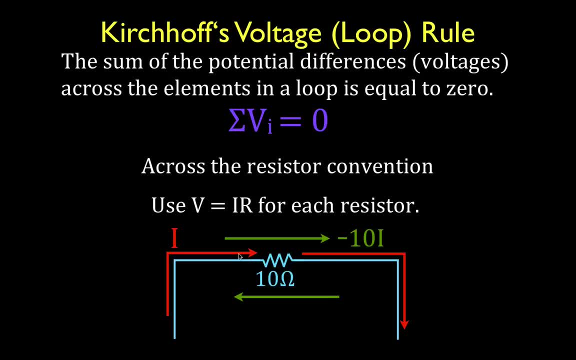 When you go against the current or upstream, then you have a potential gain. So now it's the same voltage, but the sign is going to be opposite. The magnitude is the same. Once again it's going to be: V equals I times R. 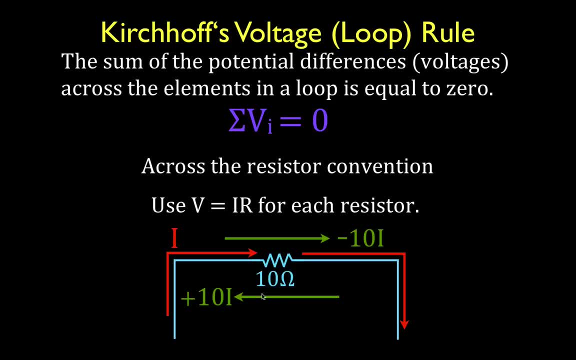 But it's going to be positive because we're going against the currents. We have to remember, if we go against the current when we go across the resistor, we put a positive sign If we go with the current when we go across the resistor.